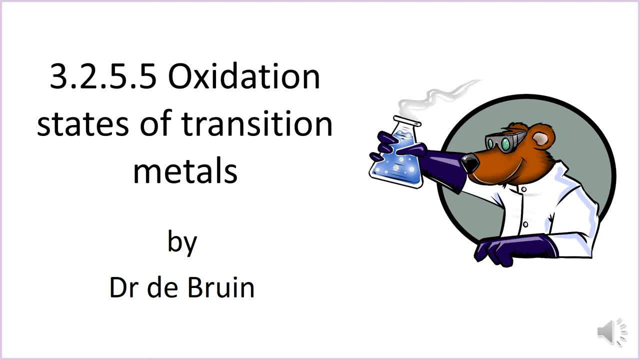 This video is the next in a series looking at the AQA A-level chemistry topic of transition metals. This video is about oxidation states, so we talk about how transition metals have multiple stable oxidation states and then, in particular, look at two key examples: the oxidation states of vanadium. 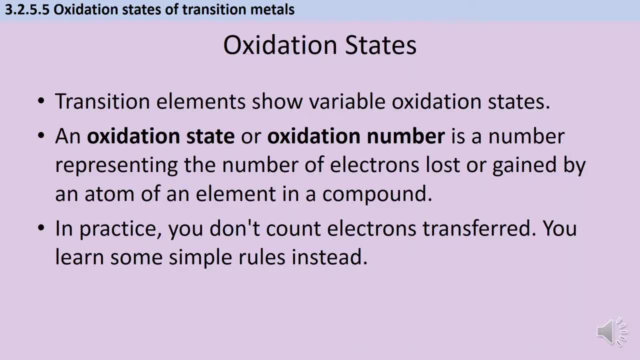 and also the silver mirror test with Tollens reagent. One of the characteristic properties of the transition metals is that they have multiple stable oxidation states. Now, you should be quite familiar with the idea of oxidation states or oxidation numbers from your AS chemistry. but if you need a little refresher, then there is a series of six videos all about redox chemistry. 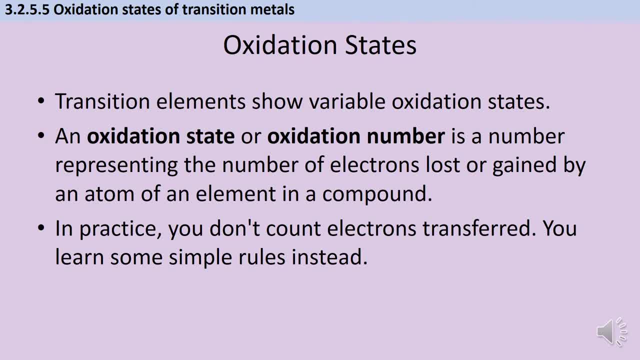 that are worth having another look at. So just as a quick refresher, when we say an oxidation state we mean it's a number that represents the number of electrons are lost or gained by an atom of an element in a compound. So in some reactions it's really obvious what's been oxidized and what's. 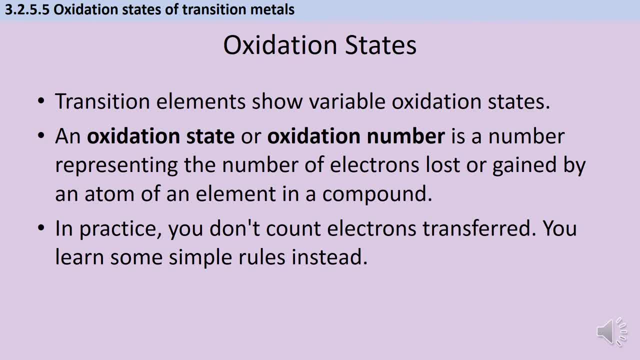 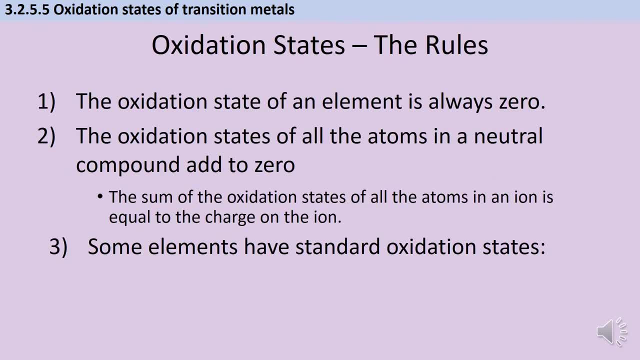 been reduced, but in others we need to do a little bit figuring out, and oxidation states are a way of numerically doing that. So in practice we don't count the electrons, we just learn some rules. The first rule is that where you have an element, 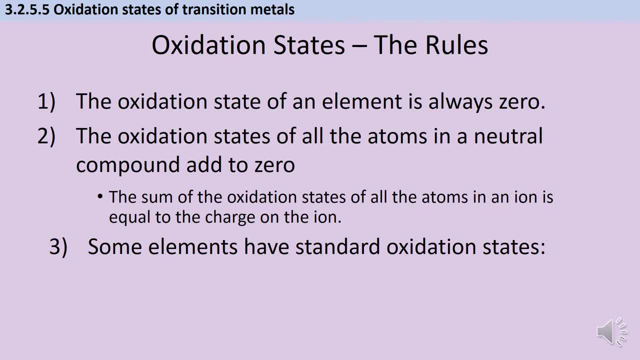 that oxidizes, it's okay to have an element of other forms of electron production. The second rule is that where you have an element that oxidizes, it's okay to have an element of other forms of electron production. oxidation state is always zero, although that's not particularly relevant when we're talking about. 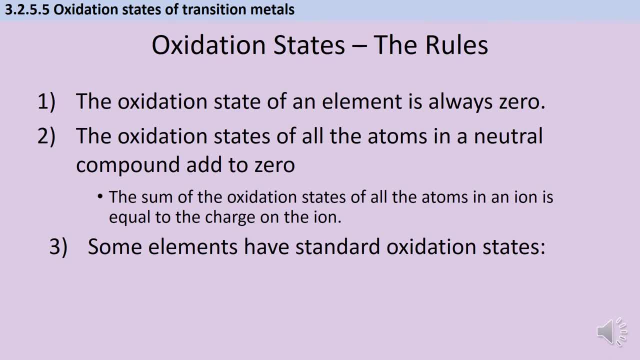 transition metals. The second is that where you've got a neutral compound, the oxidation states are going to add up to be zero. and if you've got a compound- ion rather than a neutral compound, so a few atoms are bonded together and then there's a charge over the whole ion- then in that case the 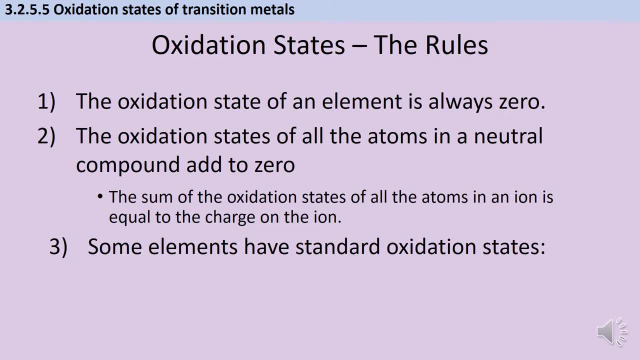 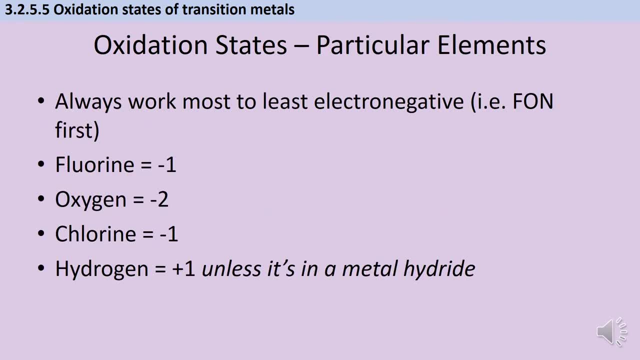 sum of the oxidation states will be the same as the charge on the ion. And then, finally, in order to help us work this out, there are some elements that have standard oxidation states. When working out oxidation states, you're always going to work from the most electronegative element to the least. 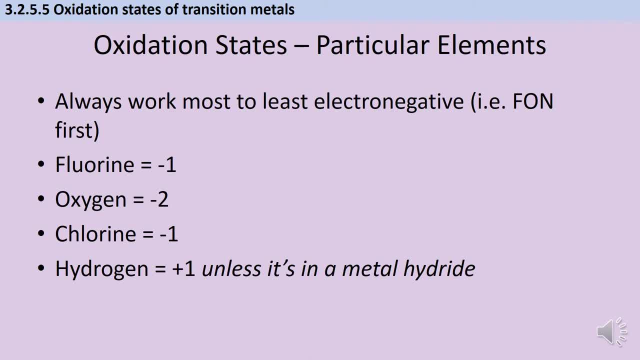 electronegative element. Now, there are more rules than this, but I've missed out all of the ones that don't apply when we're talking about transition metals. so if you need the full set of rules, go, look at the redox videos. So, in terms of transition metals, fluorine is always going to. 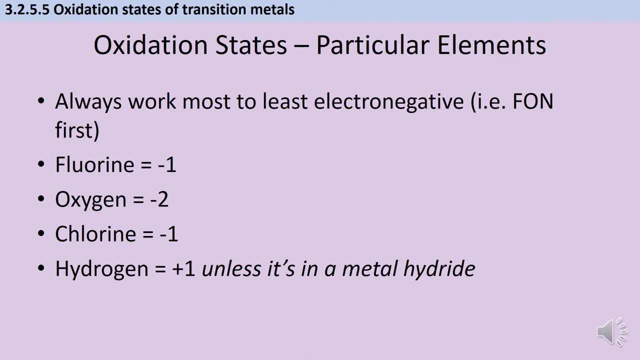 have an oxidation state of minus one. oxygen will be minus two, chlorine will be minus one and hydrogen is plus one, unless it's in a metal hydride. so actually we can ignore that plus one, because if hydrogen bonds to a transition state then it's going to have an oxidation state of minus one. So if hydrogen bonds to a 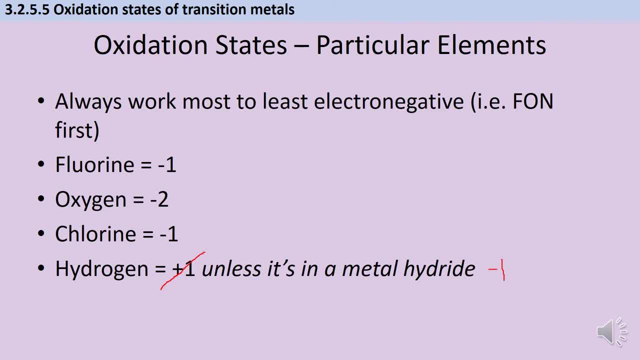 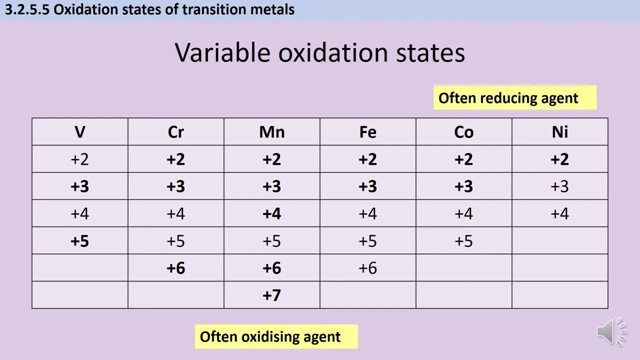 transition metal. it's going to be minus one instead. Here are some examples of the variable oxidation states of some of the transition metals in the fourth period of the periodic table. It's interesting to note that, whereas vanadium, like titanium, produces stable three plus ions, 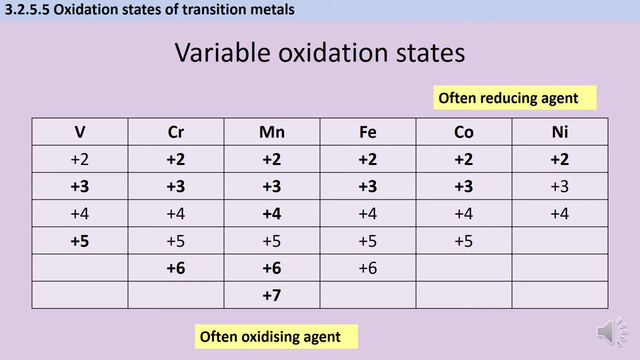 and is far less stable as a two plus ion. as we move left to right across the period, the plus two oxidation state becomes comparatively more stable, while the plus three becomes less stable. So there's kind of a general tendency for transition metals on the right hand side of that. 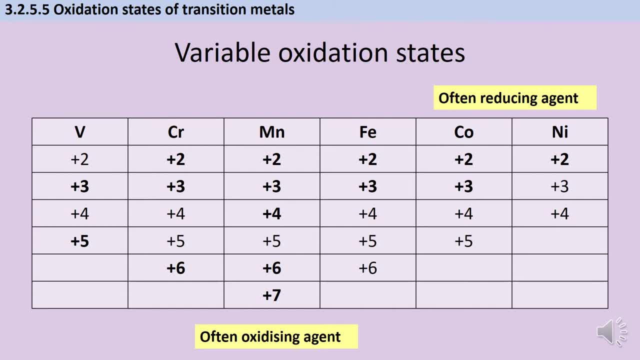 d block to form plus two ions. Another thing that's interesting to note is how these species respond electrochemically. So basically, the higher the oxidation state is, the more that species is likely to have a tendency to be an oxidizing agent. So the classic example of this are manganate. 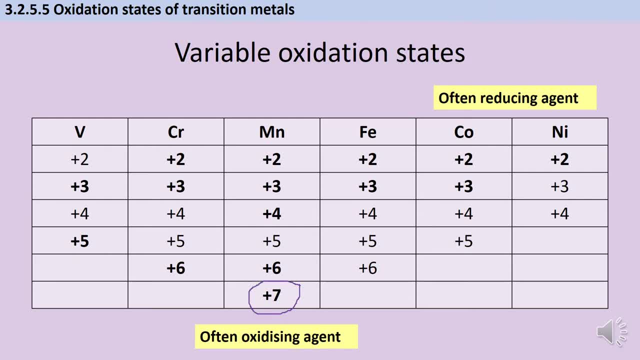 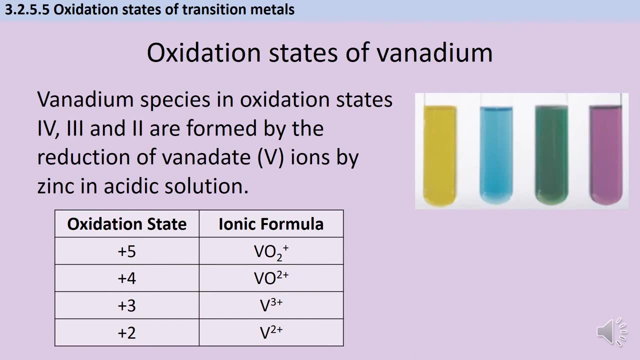 ions which contain manganese with a plus seven oxidation state, which is a really, really good oxidizing agent, Whereas other species that have a much lower oxidation state are far more likely to be good For this part of the course, AQA expects you to know about two key examples in a bit more detail. 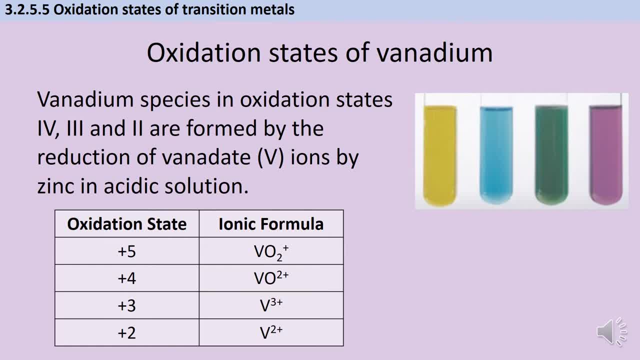 and the first one is the oxidation states of vanadium. Now we know that transition metals often have multiple stable oxidation states, but vanadium is relatively unique in that it has four stable oxidation states and each one has a particular characteristic colour when the ions are in solution. The first thing it's worth you paying attention to is making sure that you're 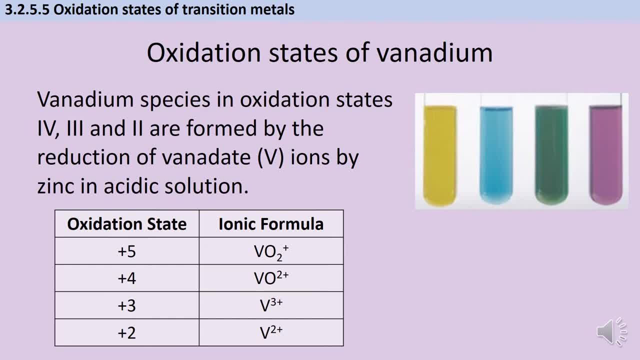 comfortable with why the oxidation state is so important. So let's start with the oxidation states, and you can do that simply by using the plus three factors and applying them to the next point. We'll start with the plus three and the plus two and you can see that these two is what it is in each 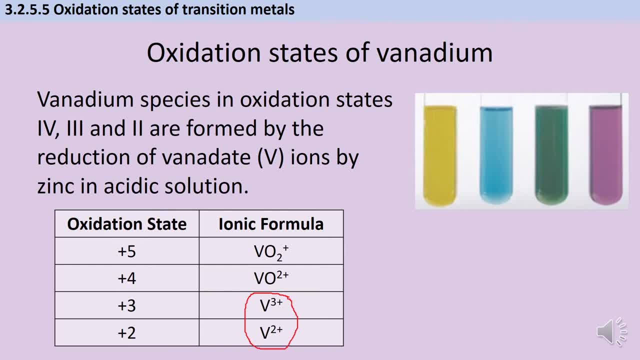 one of these ions. So the plus three and the plus two are fairly obvious because they're just monatomic ions. But let's look at these other two. so we've just said that the oxidation state of oxygen is always going to be minus 2 if it's bonded to a transition metal. and this first ion here has two. 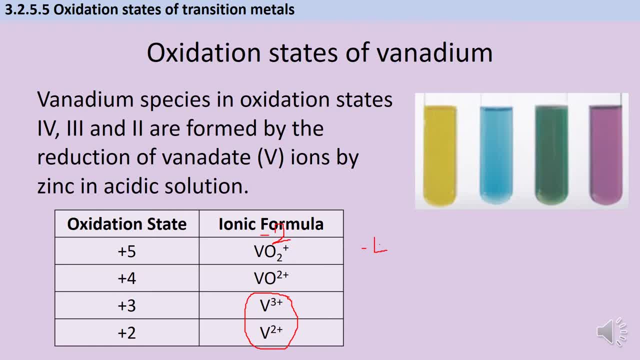 oxygen atoms in it. so that makes minus four in total, And then the overall charge of the ion is a single plus. so we then do some charging. Of course we're only going to do hydrogen nitrogen, but we're going to use the oxygen at that point because 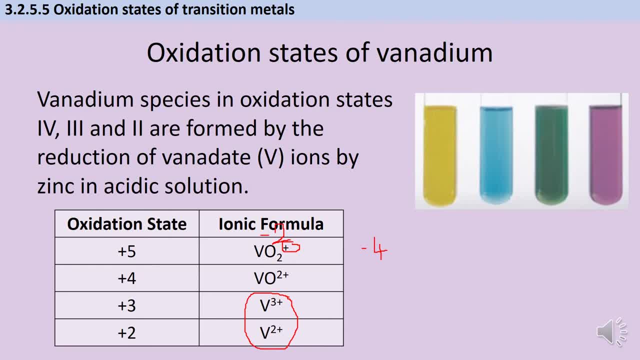 this is one of the hundreds of ions, So we're then going to find out how much is the total dose of hydrogen. So we need five pluses to balance out that minus four and the plus here, And so that's why we've got plus five here, And then in our second ion we've only got one oxygen atom, which still has an oxidation state of minus two. 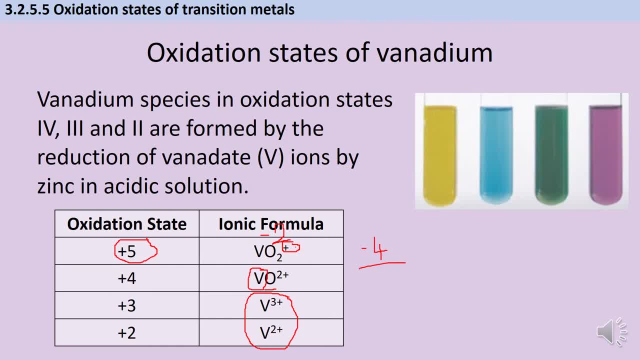 So, whatever the oxidation state of this vanadium atom here is, it has to balance out that minus two and give us enough positivity to get to two plus here, And that's why it's going to be plus four Now, as you can see, we have these characteristic colours for these different ions. 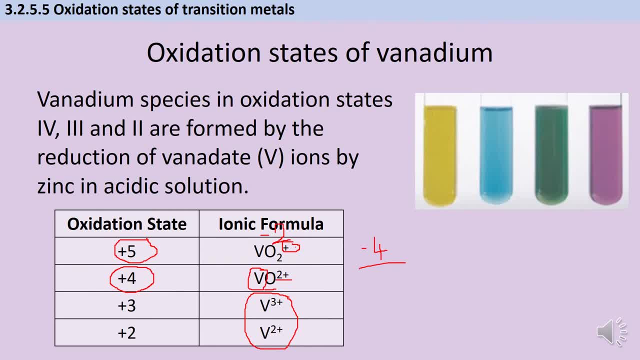 So where you start off and you have these, these first ions, these vanadium ions, with an oxidation state of plus five. then they make solutions bright yellow And then, as as that's reduced down to a plus four, the solution goes blue. Now, if you've actually done this practically, you may not have seen that blue colour. 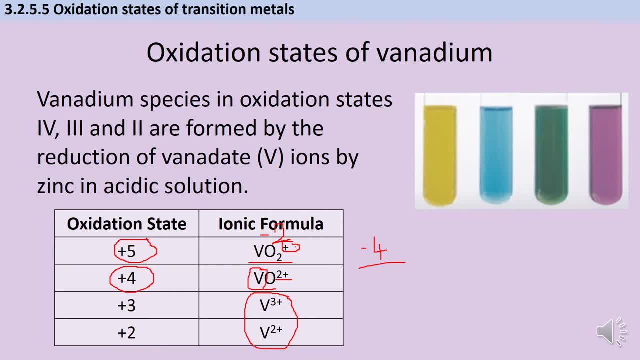 because what tends to happen is some of the vanadium is reduced and you get the blue colour, but there's still some residual yellow colour there. So quite often you just see it go a kind of greeny colour, and people end up thinking that the first colour change is from yellow to green. 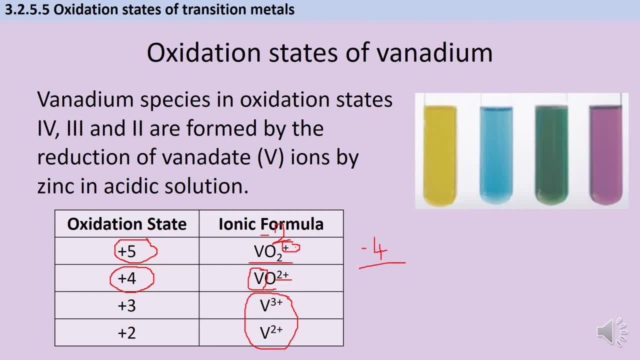 But it's not. It's yellow to blue, It's just that there's still some yellow stuff left behind. But it is possible to stop that reaction, like we've done here, so that you can see those colour changes more clearly. Then, if the zinc carries on reducing those, those vanadium atoms, then we're going to end up. 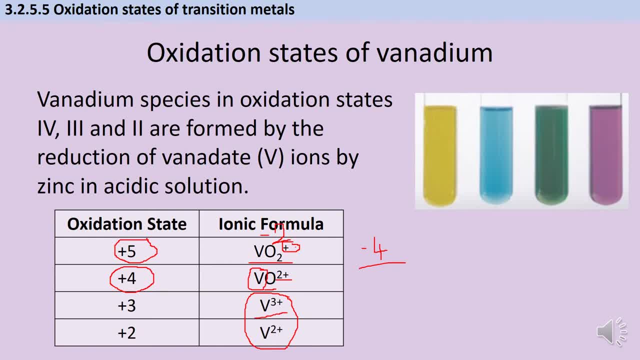 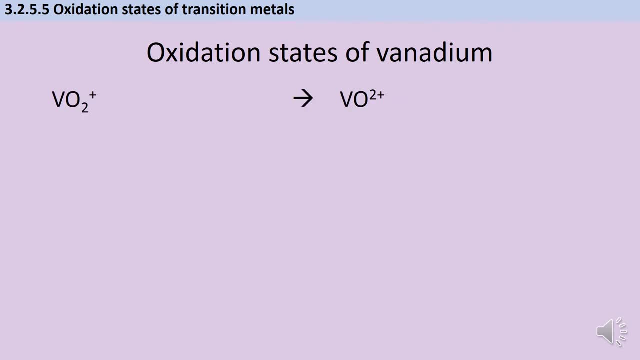 With the first monatomic ion with a oxidation state of plus three, and that is green in colour. And then, finally, we have this really nice violet colour for vanadium with an oxidation state of plus two. For each one of these reduction processes, you need to be able to write an equation describing what's happening. 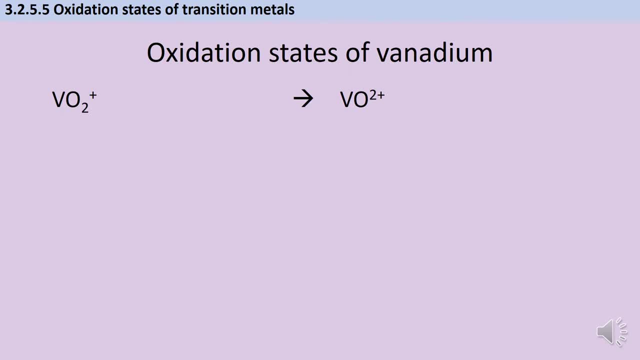 Now again, if you're feeling a little bit rusty with half equations, there is a whole video on doing those as part of the redox series. We're just going to go through these really, really quickly, the three that you need to know for the reduction of vanadium ions: 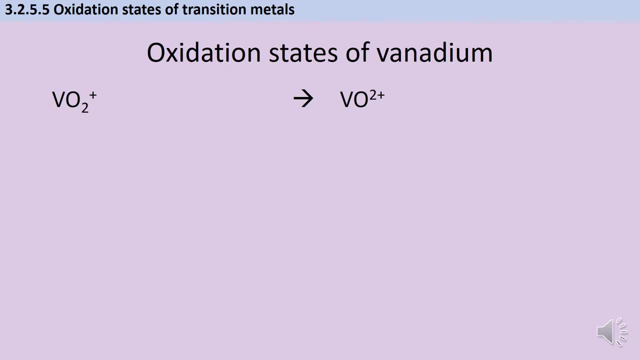 So we're going to go through these really, really quickly. So, to start with, we've got these vanadate ions over here on the left with an oxidation state of plus five, And then on the right we've got the other vanadium containing ion which has an oxidation state of plus four, or the vanadium inside it does. 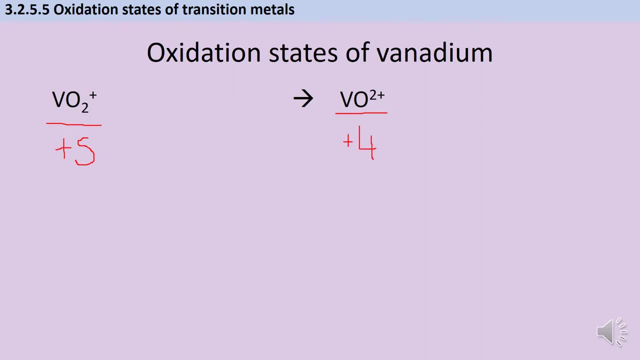 And, as you know, the first step in balancing a half equation is to check that we have the same number of atoms of the element that is changing oxidation state. So here it's vanadium, And, yes, I've got one on each side, So that's easy. 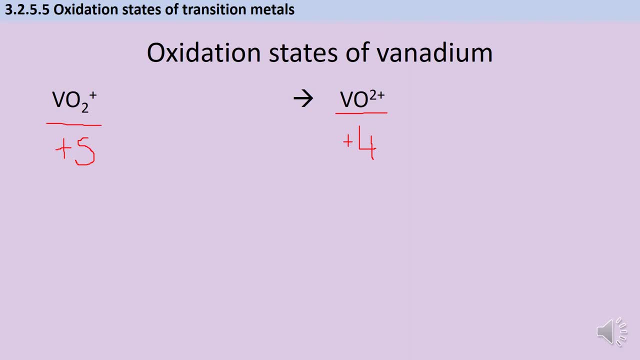 And then I can start looking at this oxygen. I've obviously got an additional oxygen on the left, but I'm not allowed to just add oxygen. That's not something I can do with half equations. What I can do is add water, So I add a water molecule to the right. Unfortunately, that doesn't just come with oxygen. 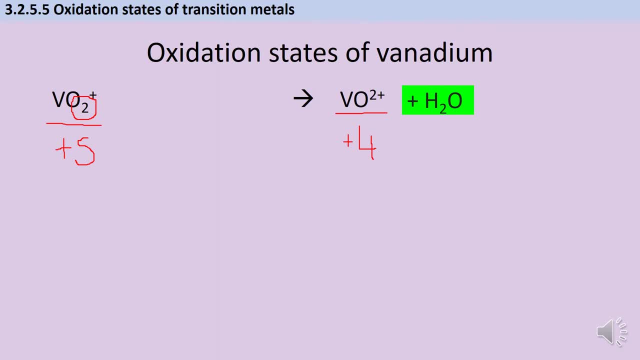 It also contributes to hydrogen atoms, So I can't balance that by adding two hydrogen ions on the left. Now, if you remember, we said that this reduction of vanadium required zinc, and then it also required acidic conditions, And this is why. 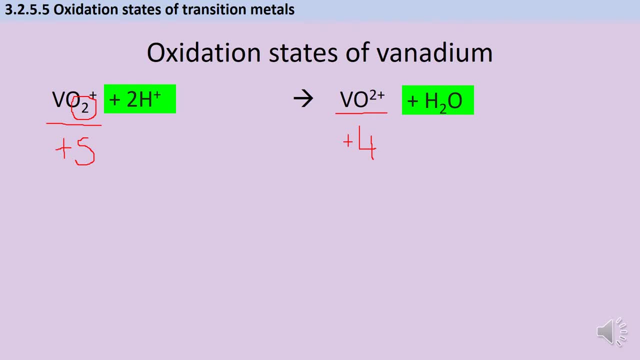 Because in order for this first step to happen- and actually the second step as well- you need hydrogen ions, and hydrogen ions, of course, make the solution acidic. Now, finally, I need to balance out the electrons. So I'm going from an oxidation state of plus five to one of plus four. 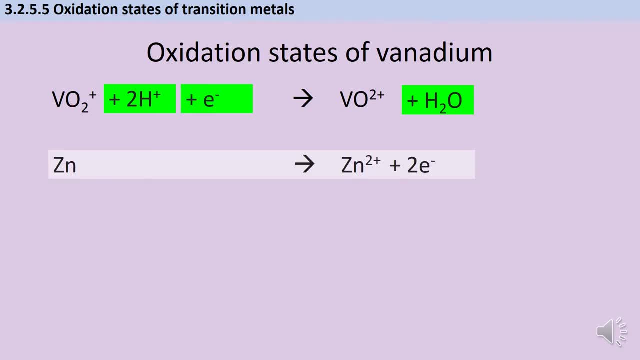 And so I'm going to need an electron here. If we're going to write a full equation rather than just a half equation, then we also need to take account of what's happening to the zinc. So while the vanadium is being reduced, the zinc is being oxidised, and it's losing two electrons. 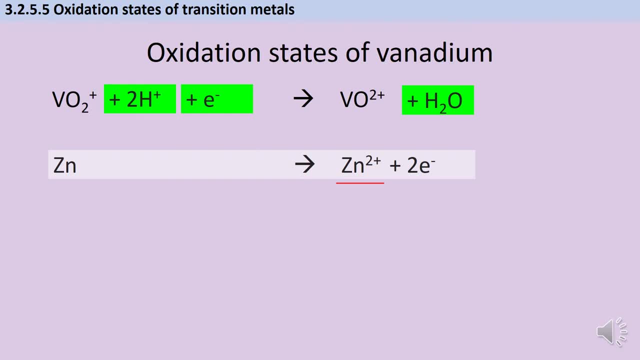 because the stable ion of zinc is zinc two plus. Now, in order to match these two half equations together and make them into a full equation, the electrons need to balance, which right now they don't. So what I need to do is take this top equation and multiply the whole thing by two. 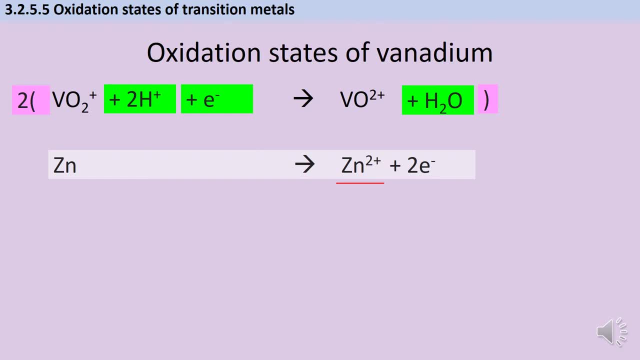 So then I've got two electrons on the left from the top equation and two electrons on the right from the bottom equation, And I can just cancel those out. So if I now match these two equations, these two half equations together, I get zinc with two vanadate ions and four hydrogen ions. 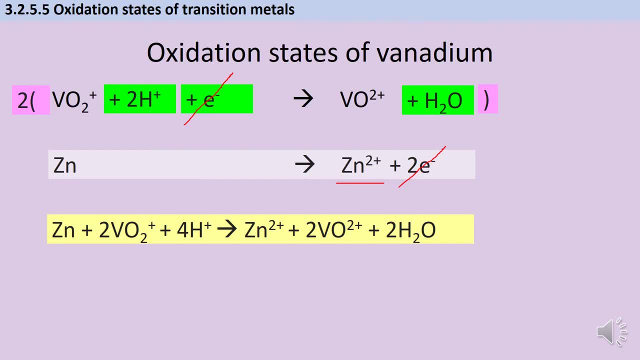 turning to zinc, two plus ions, with two more of these vanadium containing ions and two water molecules. The next part of the reduction process is very, very similar. So again I've got a single atom of vanadium on either side of my equation and the one on the right is in this monatomic ion. 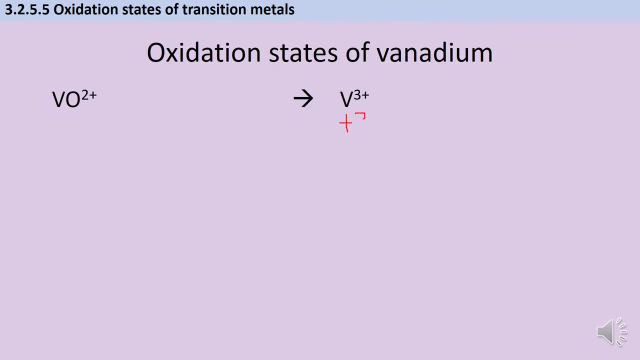 which obviously has an oxidation state of plus three, because you know it's just a vanadium ion. And then over here on the left I've got vanadium with an oxidation state, I've got vanadium with an oxidation state of plus four And again I've got an oxygen atom on the left, 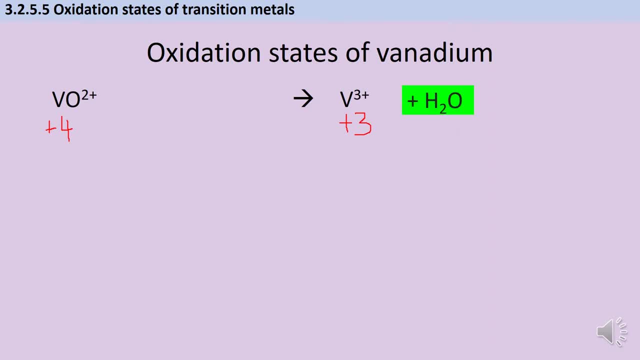 So I balance that out by adding a water molecule to the right and then two hydrogen ions to the left. So again, this needs to be done under acidic conditions, And then I balance my electrons. And then again, if I add in zinc, then I'm going to see that I'm going to need to double my top equation in order to make those electrons balance. 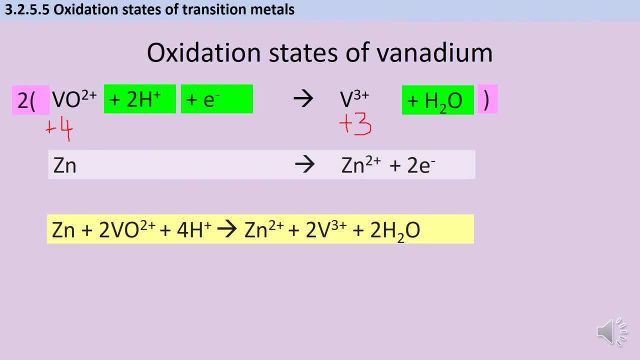 So I end up with an overall equation that looks a little bit like this, So you can work these out. You don't really need to memorise them As long as you're confident with how to write half equations. And then, in my final stage, I've got a really, really easy half equation because I've just got these two monatomic ions. 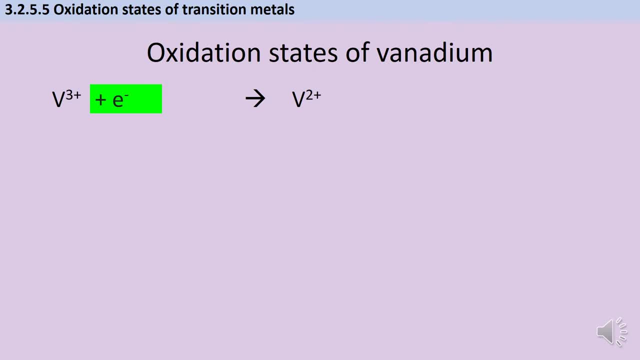 So all I need to do to balance out is to add an electron, And then again, when zinc gets involved, I need to double that top equation so that I can balance out the electrons And I'm left with this overall. So to recap, the oxidation states of vanadium: 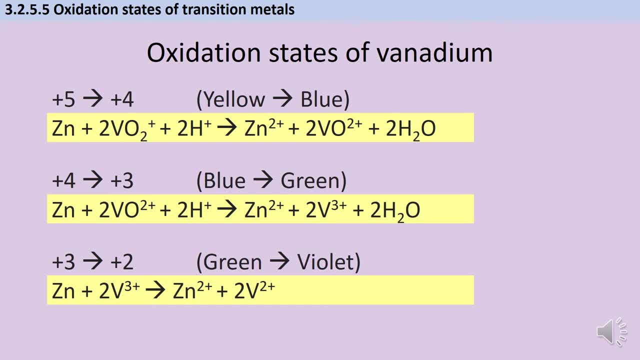 you've got a first colour change going from yellow to blue, And that happens when the oxidation state changes from plus five to plus four. Then that blue turns to green as it turns from plus four to plus three, And then the green turns from violet as the oxidation state changes from plus three to plus two. 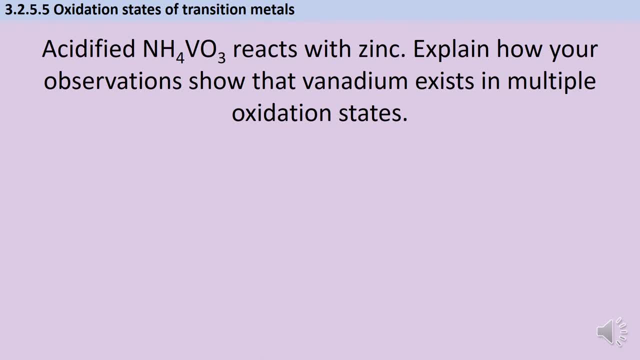 An exam question might ask you something like: acidified ammonium. metavanadate reacts with zinc. Explain how your observations show that vanadium exists in multiple oxidation states. So what we want to say is that we can see these colour changes. There are multiple colours of solution. 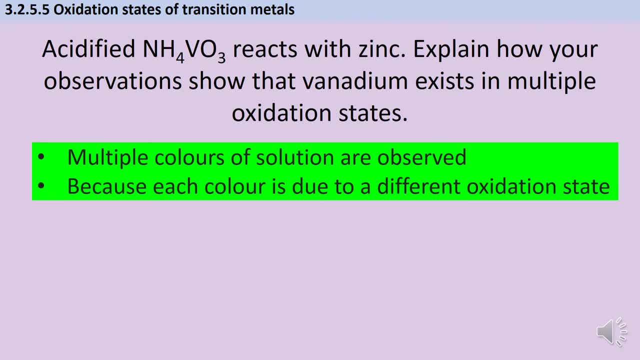 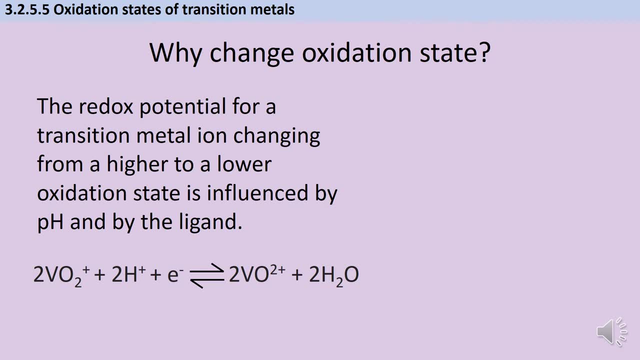 And that's because each colour of solution is dependent on a different oxidation state of the metal. You might wonder what would cause an oxidation state change in a transition metal And, as we've already hinted, sometimes reaction conditions can play a role. So, as we saw in this reduction of vanadium, you need these hydrogen ions in order for that reduction to occur. 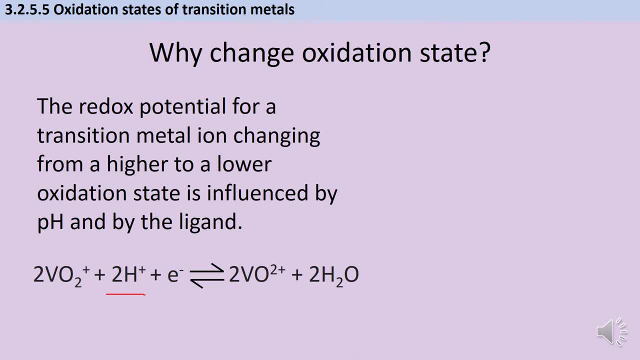 And that's very often the case. This isn't a hard and fast rule. It's not perfect And, as we said, there are some oxidation state changes that will happen independently of reaction conditions. But, generally speaking, acidic conditions are going to favour reduction. 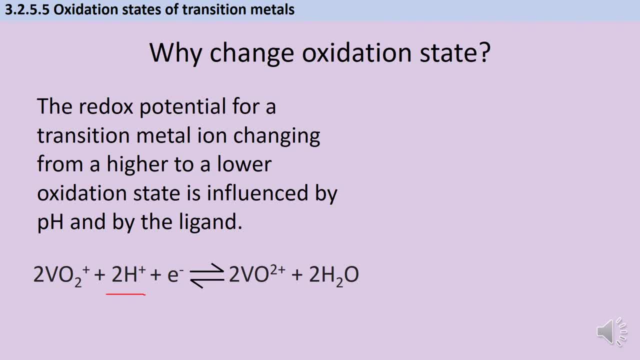 And then, funnily enough, given that they're reverse processes, oxidation is going to be favoured by alkaline conditions. So as we change the pH, it's going to affect the position of the equilibrium. So if I've got some hydrogen ions, I'm going to add in to this, this equilibrium mixture that I have here. 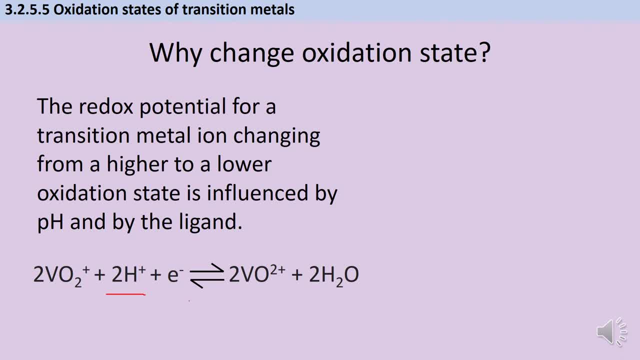 then obviously Le Chatelier's principle says that that's going to push the equilibrium over towards the right hand side, It's going to favour the forward reaction And therefore we're going to have more of the right hand ions being produced, Whereas if I added an alkali, then that would react with the hydrogen ions and remove them from the solution. 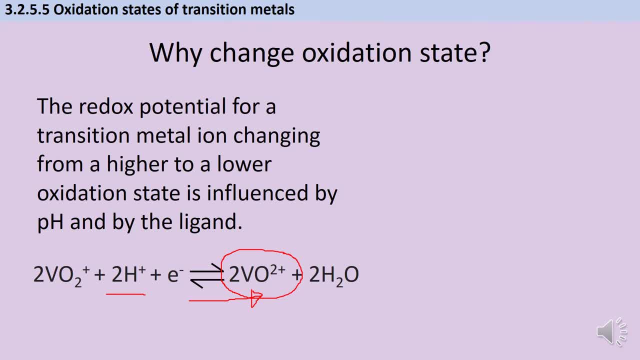 And that would then push the equilibrium back towards the right hand side. The position of that equilibrium can also be affected by the ligand that is interacting with this ion. So we're kind of simplifying things a little bit here When we talk about a vanadium two plus or vanadium three plus ion. 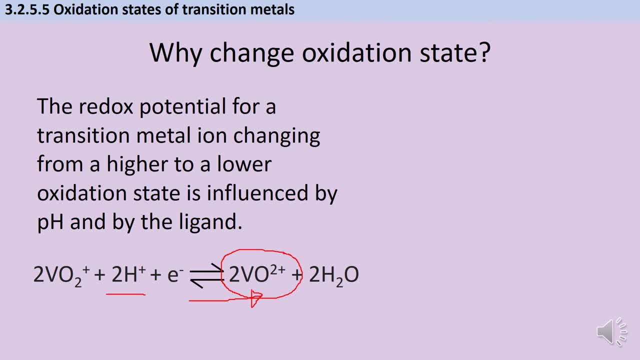 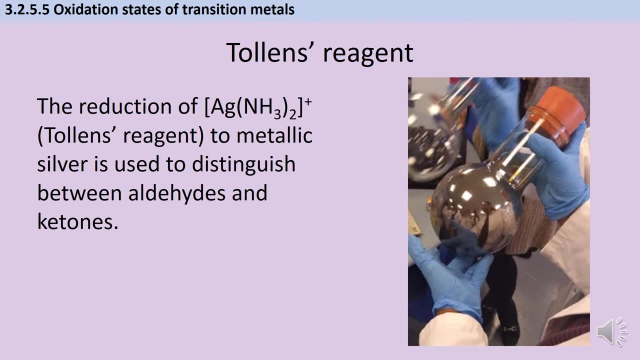 they're actually not really going to hang around as those single monatomic ions. They're going to be part of complexes, like we've seen in earlier videos when we looked at copper and iron, two and three, plus and also cobalt. The next reaction that you need to be aware of for this part of the specification is the use of Tollens. 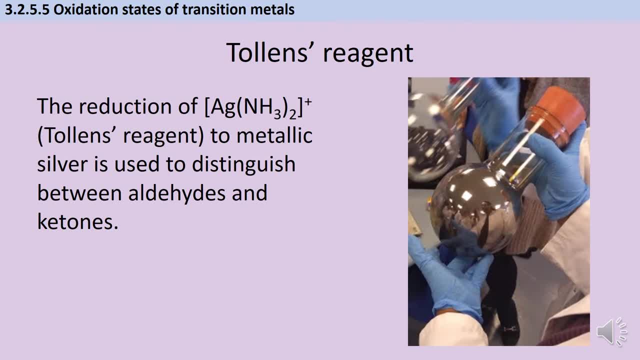 reagent to distinguish between aldehydes and ketones, And this is a reaction that you would have met during your year 12 organic chemistry. So to make this, this Tollens reagent, we take some silver nitrate solution and add a tiny amount of sodium hydroxide. 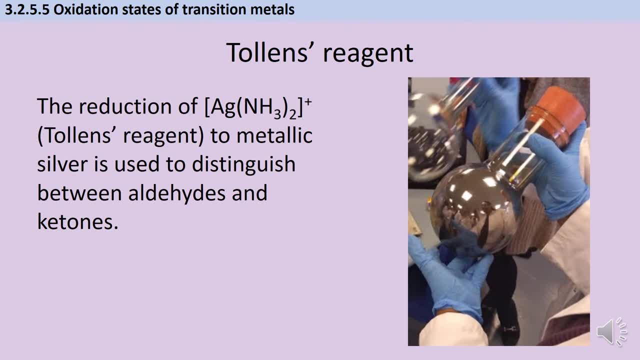 which is going to make it slightly alkaline and that's going to cause a precipitate of silver oxide. And then you add enough dilute ammonia to redissolve that precipitate and you make this diamine silver ion Now, because the solution is alkaline. 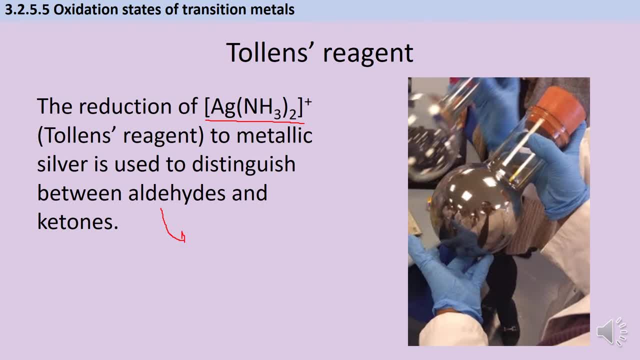 it's possible for this aldehyde here to be further oxidised to make a carboxylic acid, or at least to make a salt of the carboxylic acid. And that doesn't happen if you've got a ketone, because it can't be oxidised any further. 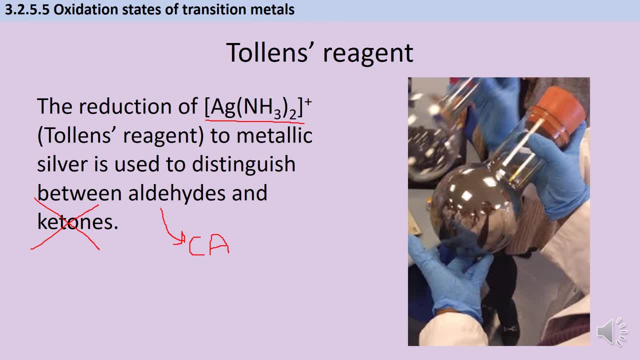 So as the aldehyde becomes oxidised to make the carboxylic acid, then the silver is going to be reduced, It's going to pick up an electron And, rather than being a silver ion, we're going to have atomic silver, which is obviously then not soluble.